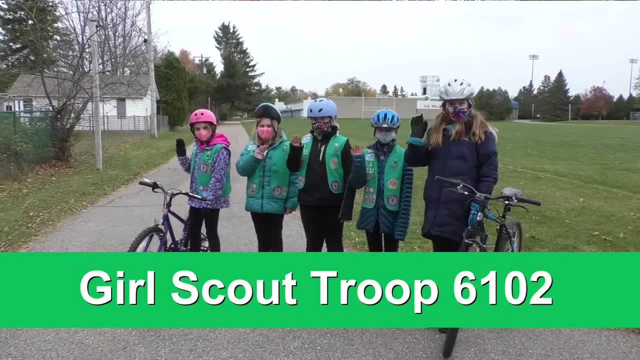 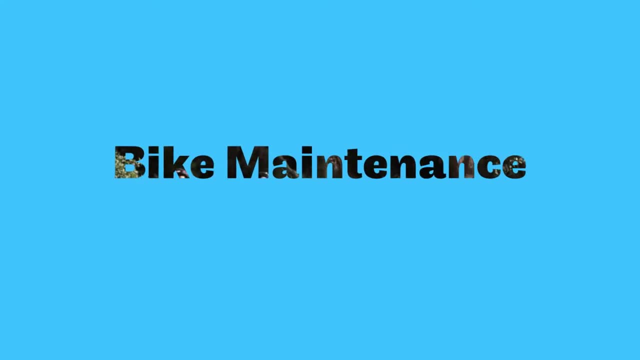 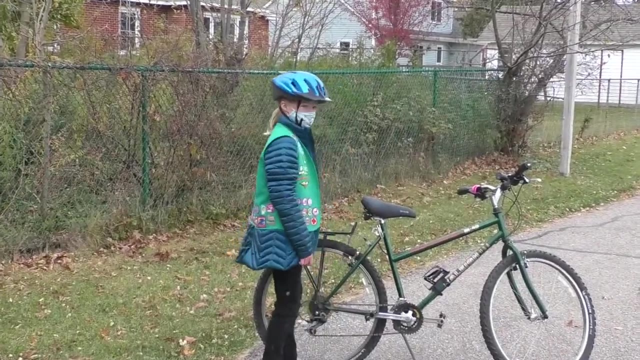 Hi, welcome to Bike Safety 101 with Troop 6102.. My name is Elizabeth and our lesson today is learning about bike maintenance. The first part of a bike we need to check is the seat. Check your seat to see if it's tight. Make sure it doesn't move side to side or up and down. 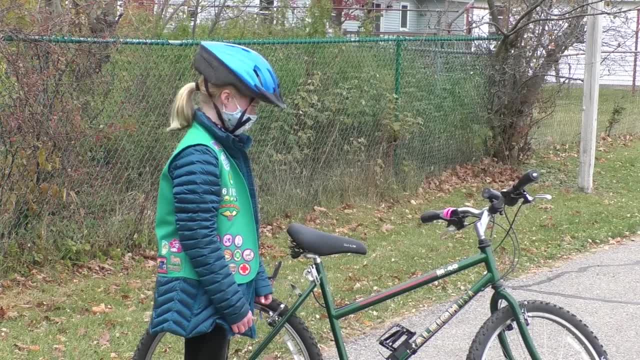 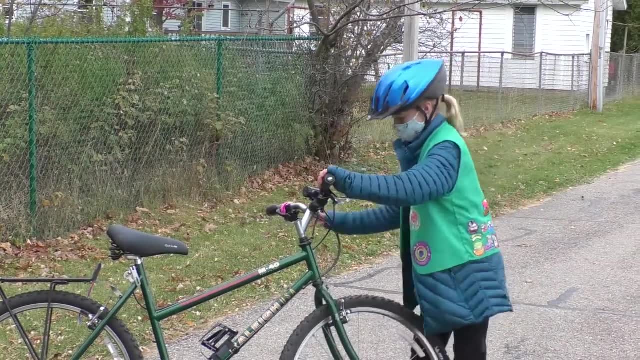 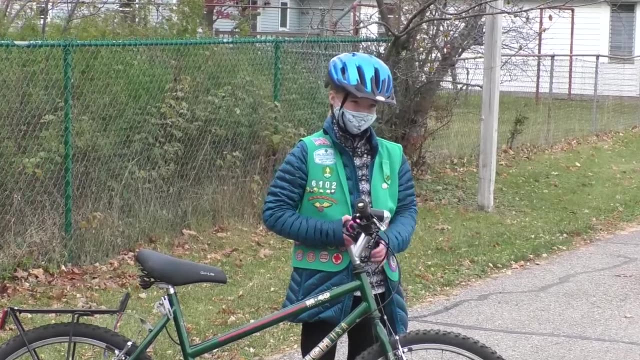 Next we'll check the handlebars. Check that the handlebars are not crooked or loose. You should not be able to twist them back and forth when you hold your front tire between your legs. Brakes: Check your brakes to see if they work by squeezing your brakes to make sure. 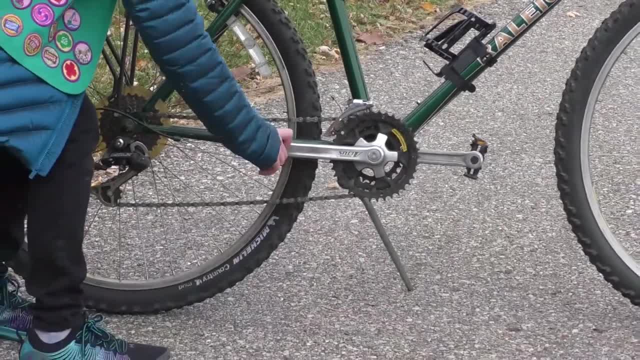 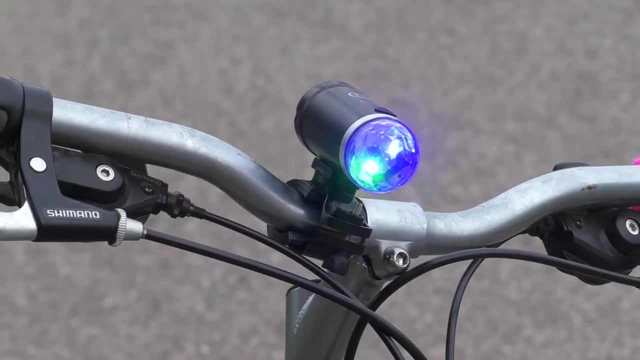 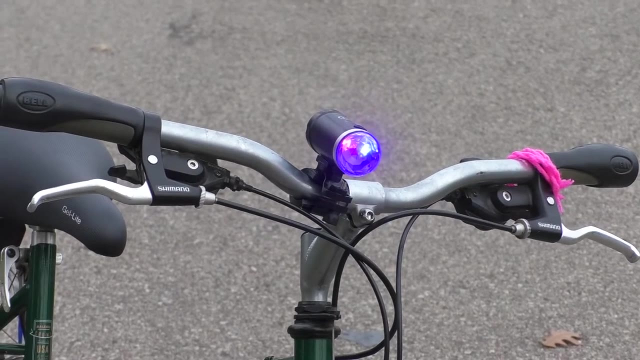 the tires, stop moving. Pedals: Make sure your pedals are tight and spin smoothly. Lights: Make sure you have working lights on the front and rear of your bike. If you ride in the city of Stevens Point at night, you need a front light. 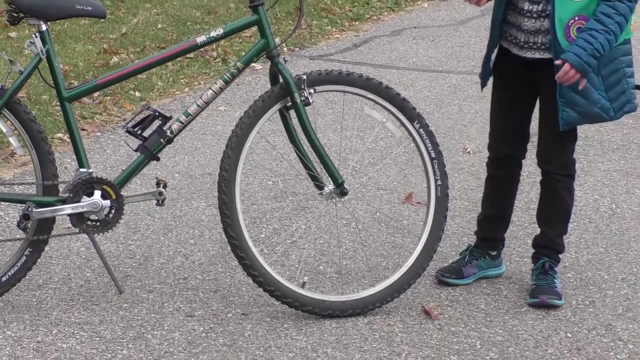 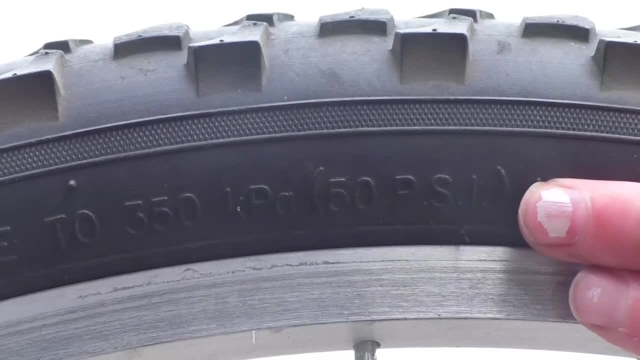 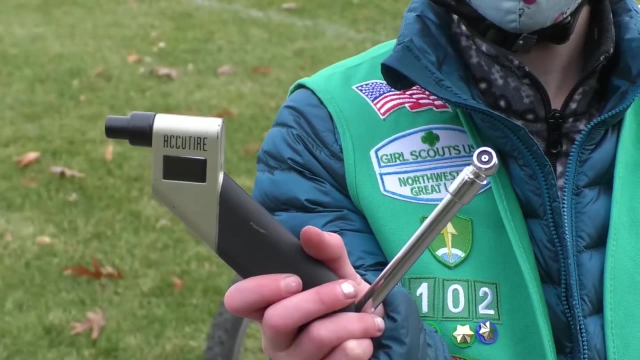 Tires. Check the tires for cuts, cracks and tire pressure. Look on the side of your tire- there are numbers in the letter PSI that tell you how much air pressure should be in your tires. Use a gauge to check If the pressureik on this. 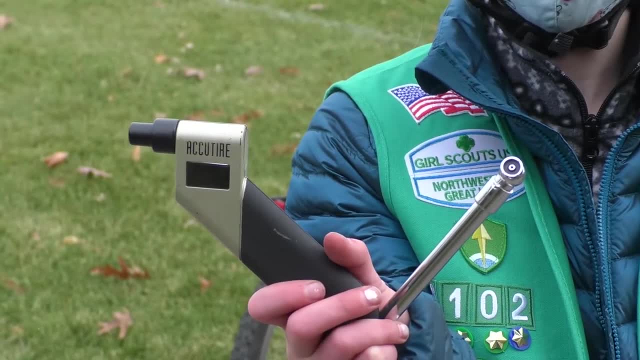 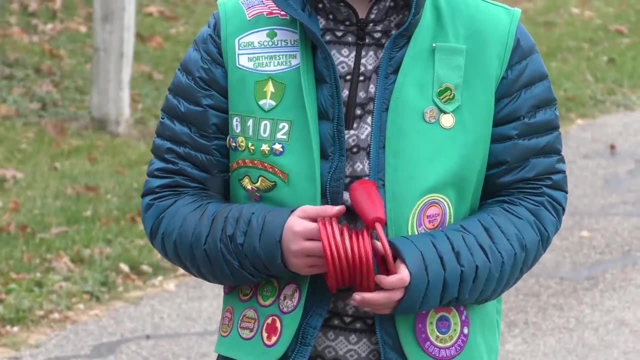 If the pressure is lower than the number on the side of the tire, that means you need air in your tires. Bike Lock: Before you head out on a ride, make sure you have a bike lock, just in case you need to leave your bike unattended. 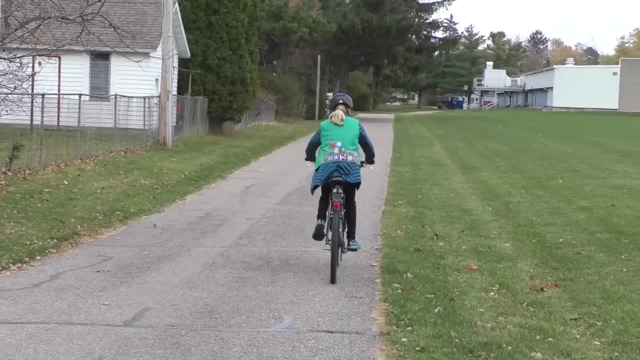 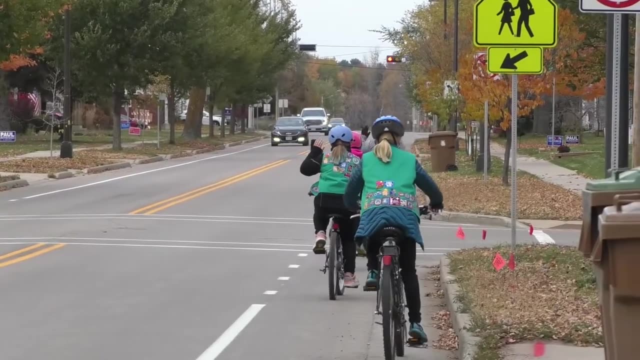 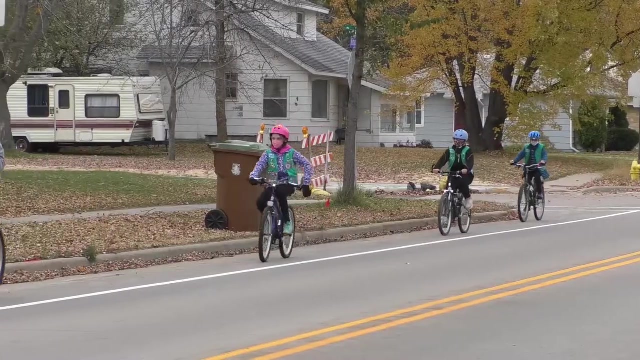 Thank you for joining us today for Bike Safety 101 with Troop 6102.. Please remember a bicycle is not a toy, it is a vehicle. So please make sure you always follow all traffic signs, laws and signals. Don't forget to use the bike lanes and remember to stay safe and have fun biking.